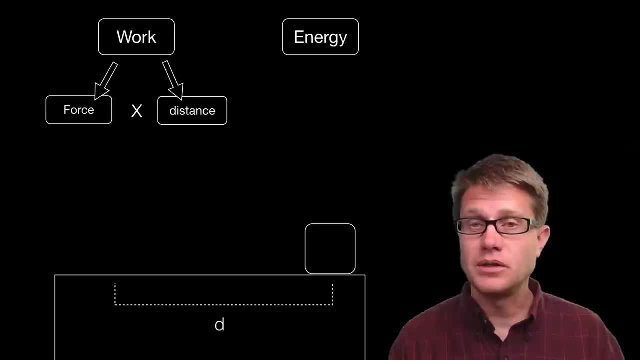 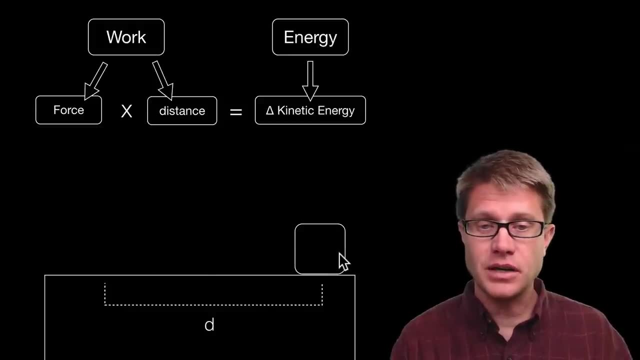 constant force over a given distance, And so we did work. Now, what is neat is that is equivalent to the amount of energy that was given to that object. This object now has kinetic energy. Now, if we wanted to figure out that kinetic energy, we could break it down into the final kinetic energy, which is socu 1, half mv squared. 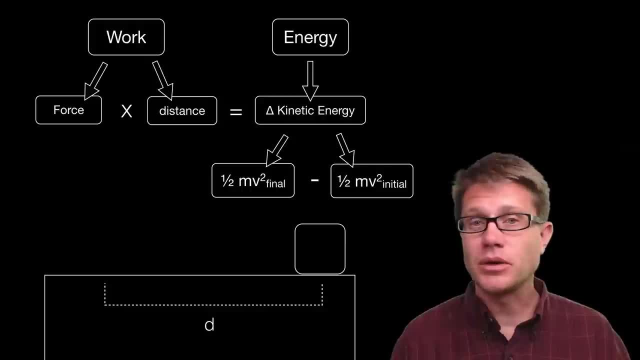 squared minus the initial kinetic energy. But what is neat is, if we just know the force and the distance, we have already figured out the amount of kinetic energy that is being added. Now let's work qualitatively for a second. Have we added energy to that object? 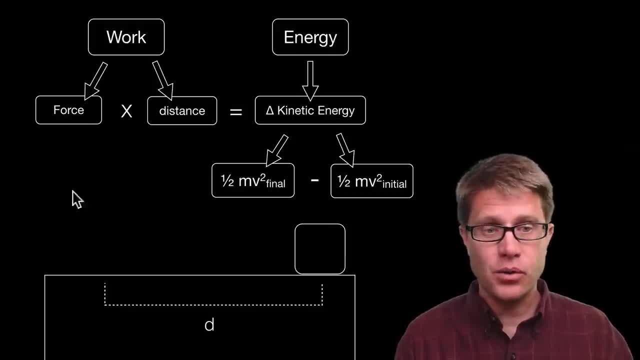 or have we taken it away? Well, since we applied a force to the right over a given distance, we know that the work is going to be a positive value. How else could we figure this out? Well, if we look at its initial kinetic energy, since it had a velocity of zero, then we know: 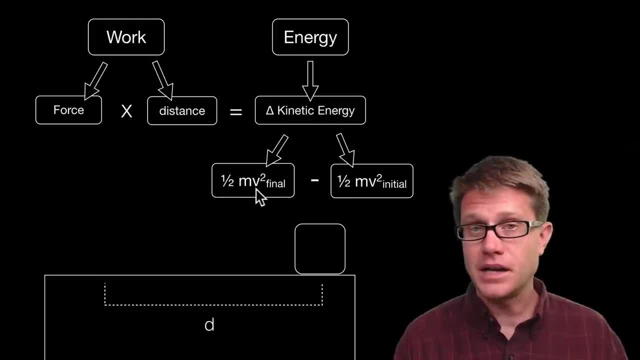 that this is a zero value. And if we are taking a value of a velocity minus a zero value, we know this is going to be a positive value, And so you can look at either the force, where the force is being added over time, or the change in the velocity and that is going to. 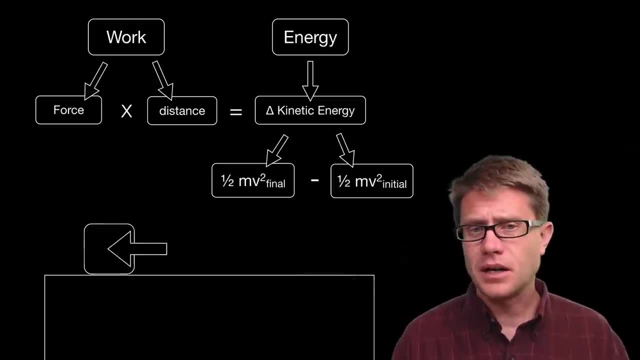 tell you if energy is being added or is it being taken away. Let's look at a different scenario. Now we have an object that is moving towards the right, and so when I start it, it is going to be moving to the right above its instagram, and I was slice right here. 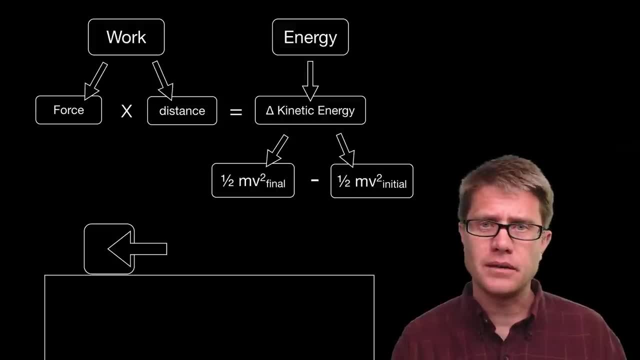 moving towards the right. But let's say we are applying a net force to the left. What is going to happen here? You can see it is going to slow down, And so what is happening to the amount of work? Well, we have got a negative force times the distance, And so 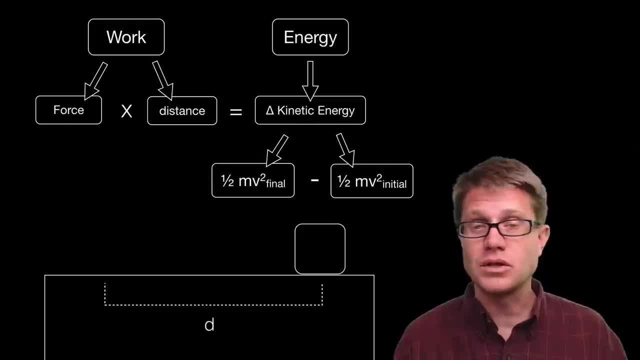 we are decreasing the amount of kinetic energy in that object. We are taking that energy away, Which makes sense because the object is coming to rest. If we wanted to look at the velocities, we could see now that we have a final velocity of 0, so this is a 0 value. 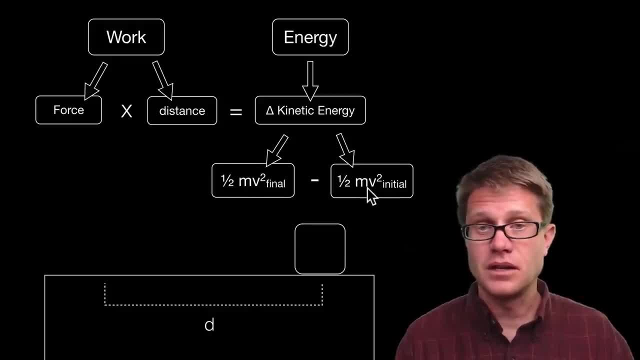 right here, minus that initial velocity, And so you can see that we are going to have a negative energy. We have lost energy, We have lost kinetic energy. Now it is not as simple as that, Because sometimes you are going to apply a force and it is not going. 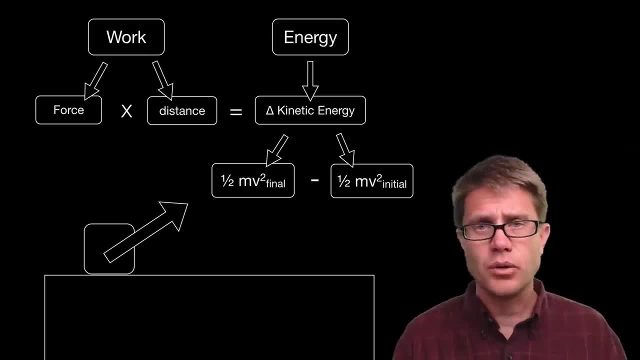 to be in the same direction as the motion. And so let's say we are pulling on that object, So you could say we have a rope tied on to it And we are moving it in that direction. Okay, now, since we have moved it in that direction, we have to break down that force vector into 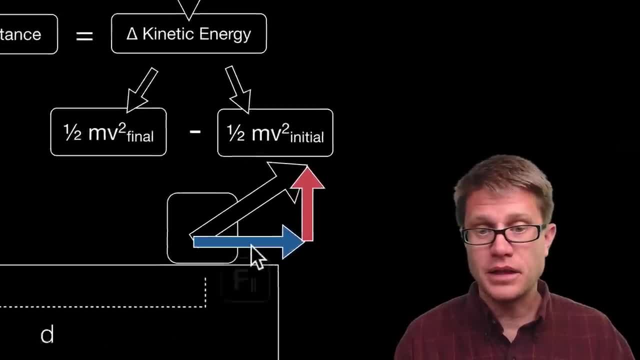 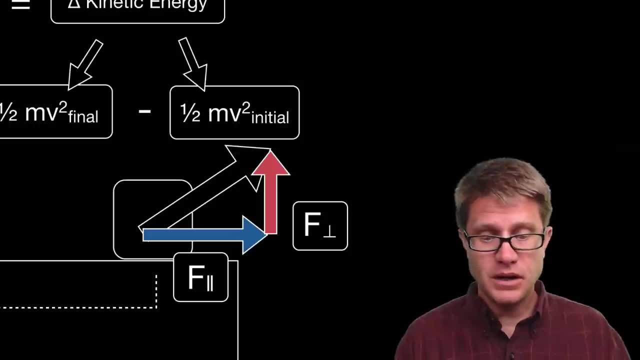 its two components, Component vectors. We have this. we will call that the force parallel. So it is in the direction of the motion, And then we have this, which is going to be the force perpendicular. Now what is interesting is that it is only this force that is acting in the direction. 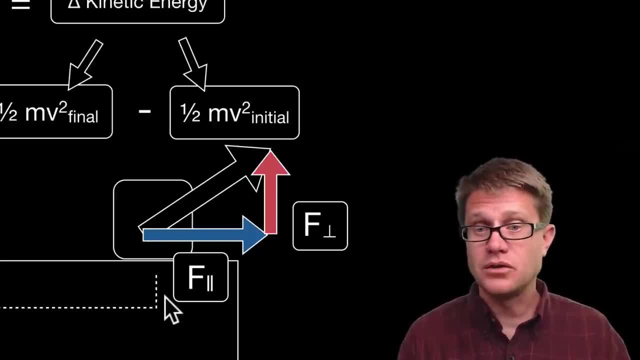 of that motion And therefore it is only that force that is doing work. The other force is not doing any work, since the motion is not in that direction. And so lots of times when you are solving problems it is not as simple as figuring out the work You have. 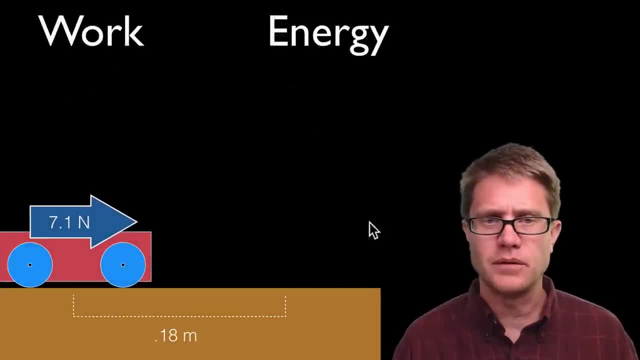 to break that force down into its components. And so what we are going to do is we are going to break that force down into its component force, And I will show you an example of that. And so let's start simple. Let's say we have a cart And that cart is moving from. 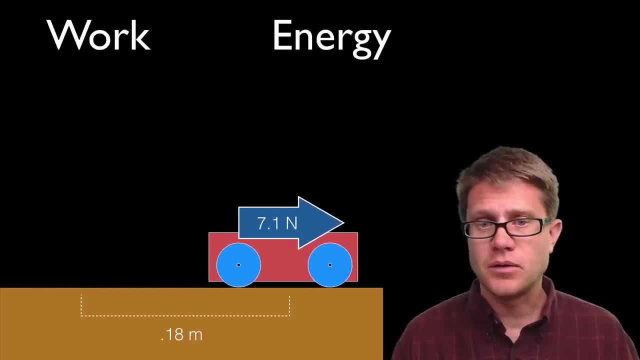 the left to the right And we are applying a constant force of 7.1 newtons. So how would you figure out the work on that cart? It is really simple. You just say work is equal to the force parallel. Again, it is going to be in the direction of that motion times the 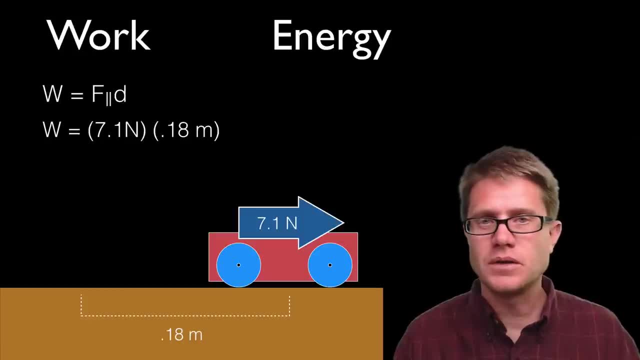 distance, And since we are given a force of 7.1 newtons times the distance of 0.18 meters, it is really simple to solve for. So what is going to be our work? It is simply going to be 1.3 joules. Now, that is the amount. 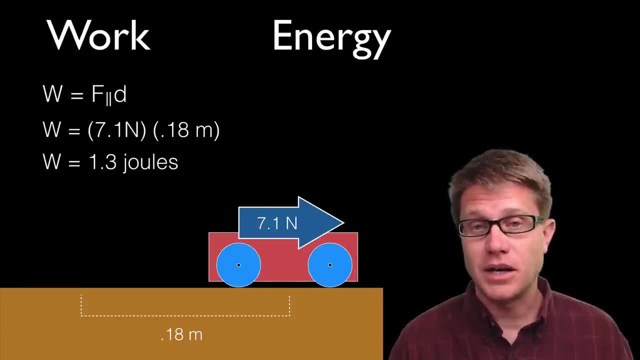 of work that was done on the cart. What is neat is it also shows us the amount of kinetic energy that was added to that cart. We do not have to figure out the mass and the velocity and initial velocity. We know by the amount of work being applied to it that that is going. 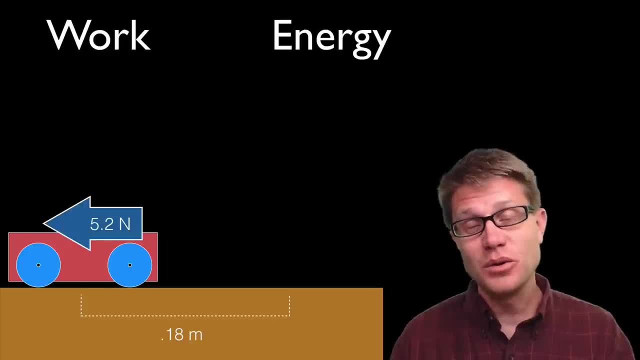 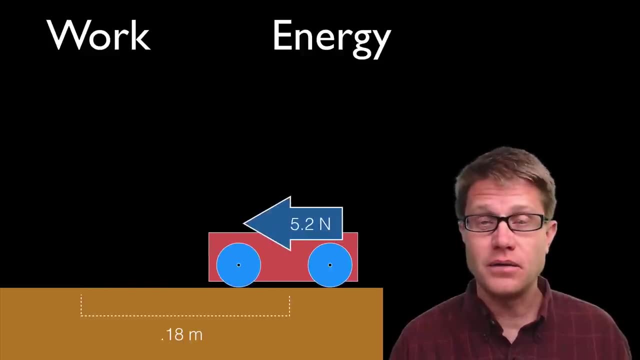 to tell us the amount of kinetic energy added. Let's look at a cart that is already moving towards the right. We are applying a net force to the left And watch what happens here. Again, it is slowing down, So how do you figure out the amount of work on that cart? Well, 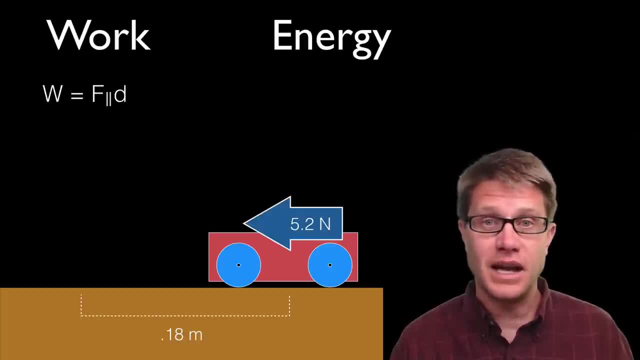 again, it is force parallel. In this case it is anti-parallel, It is in the opposite direction, And so we have to put that in as a negative value, And so we are going to have negative 0.93 joules. In other words, we are taking energy away, We are doing negative. 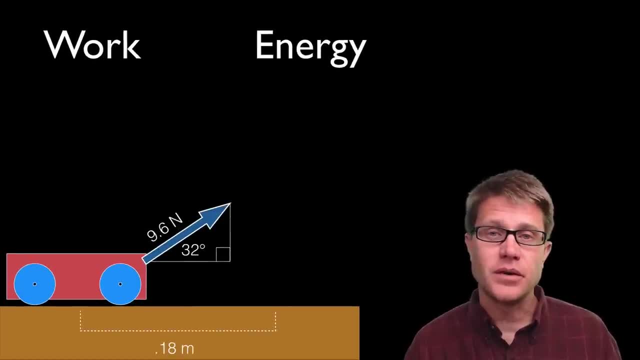 work on that object. Now let's move that force in a different direction. This makes the problem a little bit harder. You can always pause the video and try to work this out. But let's say we are applying a 9.6 newton force in this direction, but it is 32 joules, So we 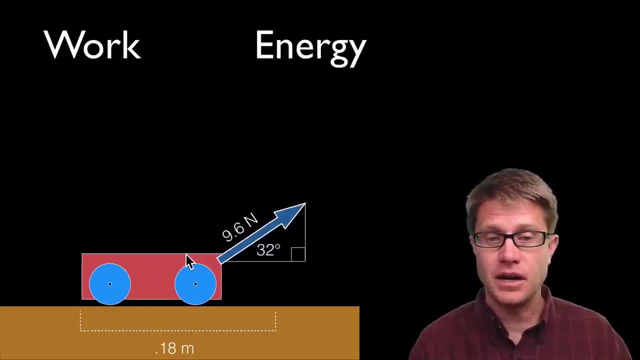 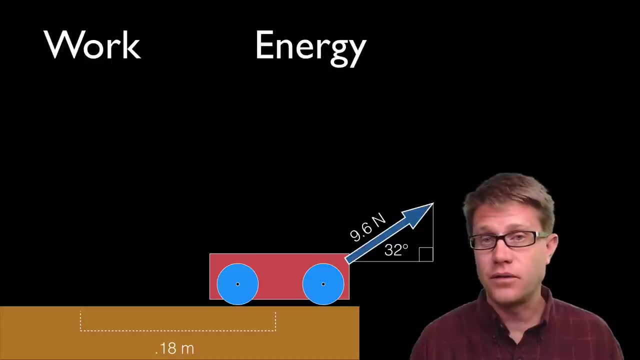 are 32 degrees up from parallel And watch what happens to that object. So it is moving in that direction. So if I want to figure out the amount of energy that is added to that cart, all I have to do is figure out the force: Force parallel times the distance. 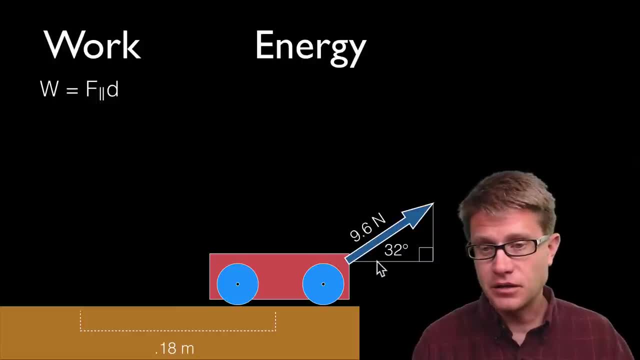 What makes this problem a little bit harder remember is that we have to target this, which is going to be that force in the parallel direction. How do we do that? Well, we just use a little bit of trigonometry, Since you know this angle and you know the hypotenuse. 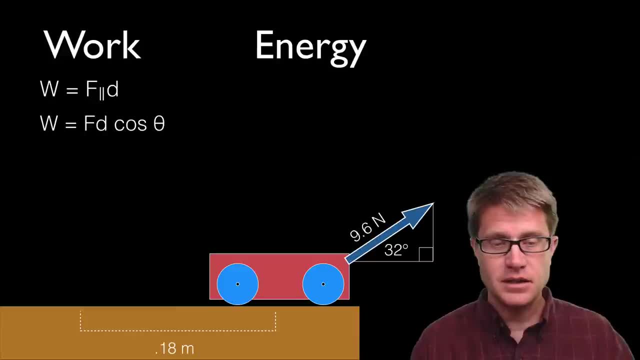 we can figure out this adjacent, And so to figure out that it is simply going to be the force times the distance times cosine of theta. What is cosine of theta? It is the cosine of this angle right here, And so that is going to. 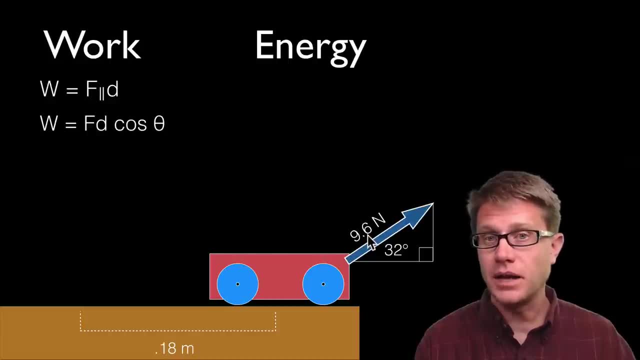 give me a force And I can always check that It should be a value that is going to be less than the hypotenuse or less than 9.6 newtons. So if I plug that in my calculator I can find the cosine of 32.. And the cosine of 32 is 0.848.. So it is decreasing that amount of. 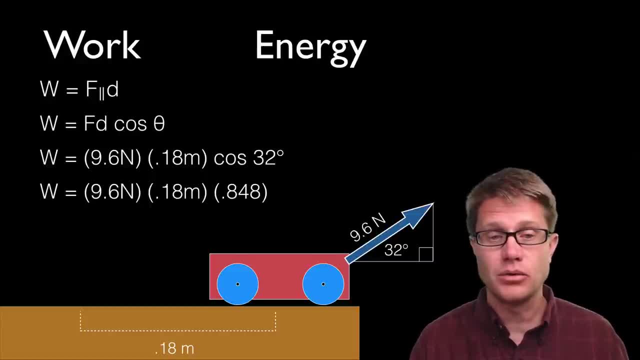 force, But it is the force that is actually moving in the direction of that motion. So now I just simply add or multiply all those values and I get 1.5 joules. Again, I am solving for significant digits here, And so how much work is done on the cart? 1.5 joules? How? 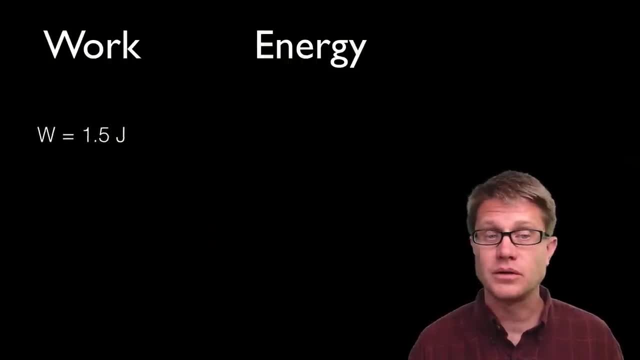 much energy has been added to the cart, 1.5 joules. And so you know, there is that equivalence. The amount of work done on that cart is equal to the amount of energy that that cart has gained, which is kinetic energy minus initial energy. And so, if you wanted to, if you were, 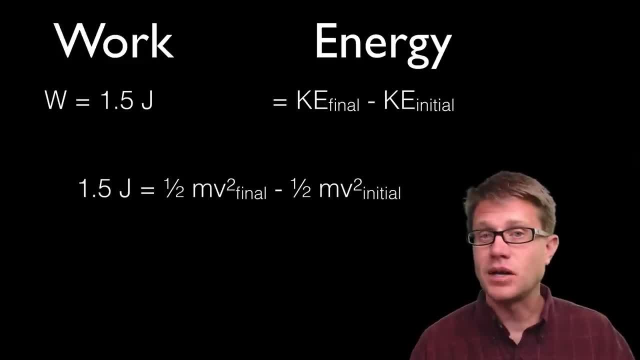 given the mass of the object, you could plug that in. Since that object is going to be accelerating, we could say that its initial velocity is 0. And so you could figure out its final velocity. And so, again, work and energy are going to be equivalent. How did 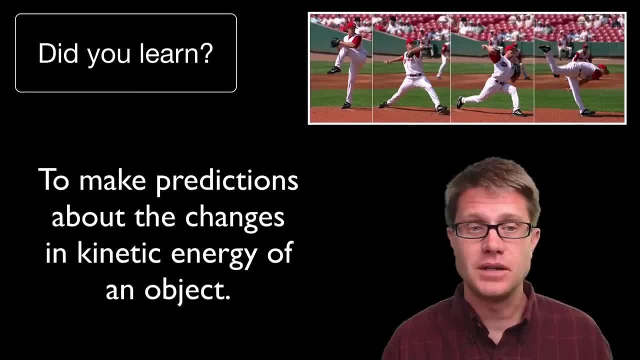 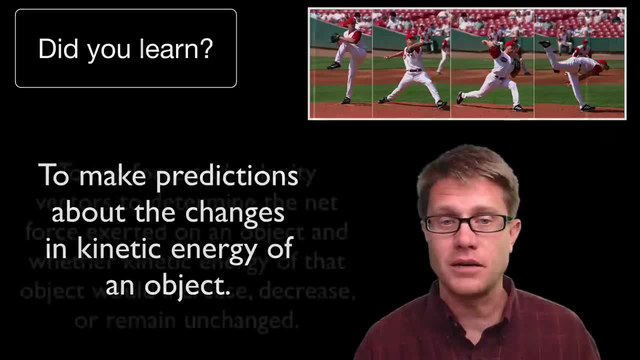 it get the energy. We applied a certain amount of force over a given distance, And so did you learn to make predictions about the changes in kinetic energy of an object. Again, if it is moving faster, it is going to have a higher amount of kinetic energy. Can you use the